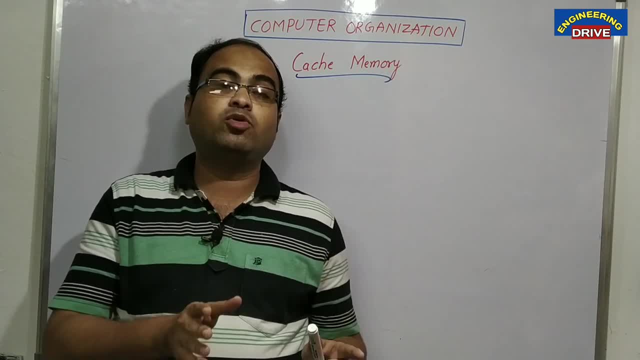 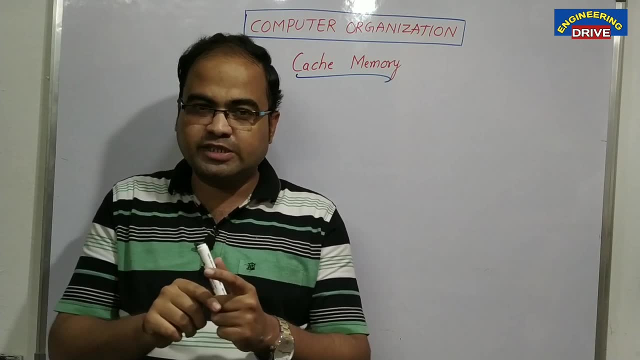 Our CPU won't execute entire program at the time. our CPU will execute instruction by instruction. However, system will explain to that system, ETC, all the parameters per mah. output is only. this is very, very important. once first instruction is executed, it will execute second. 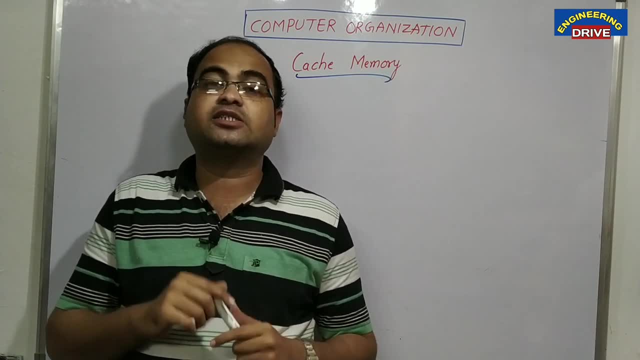 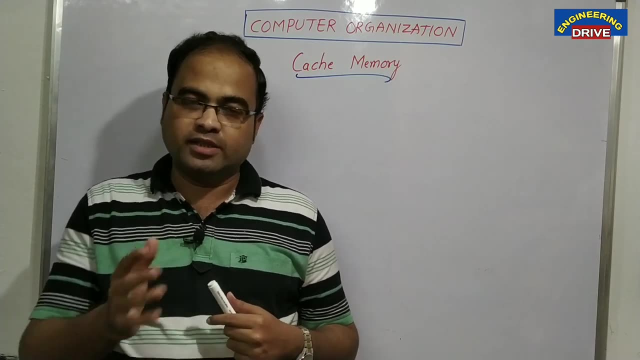 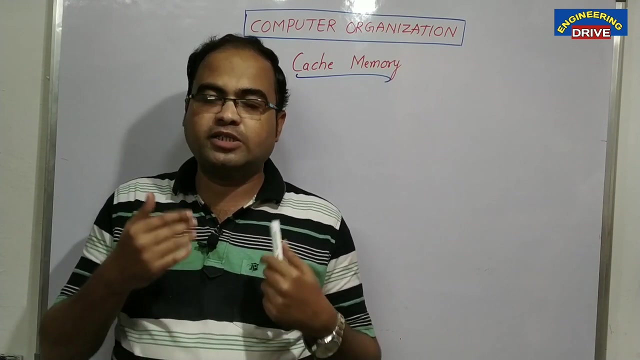 then third, then fourth. we call this cycle as instruction cycle. already i have explained to you in my previous parts- if you have not watched, you can go ahead and watch that. okay now- what is the role of cache memory in the execution of those programs, or execution of those instructions by the. 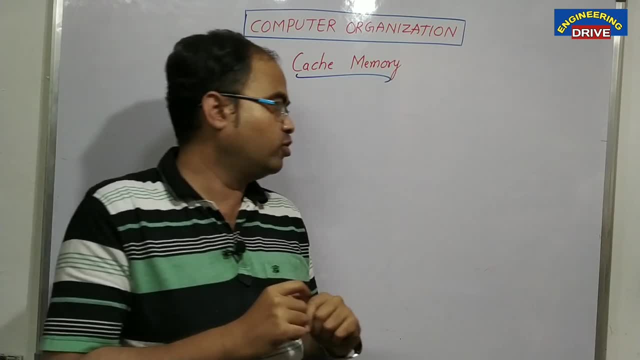 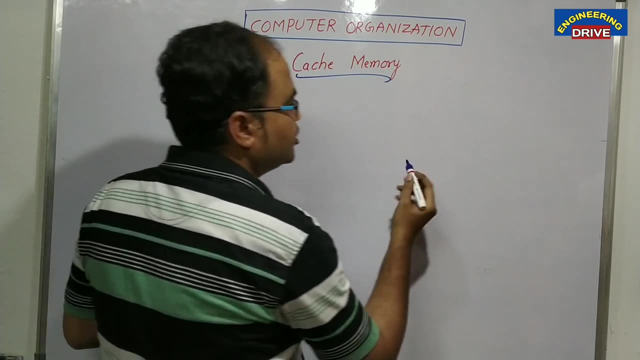 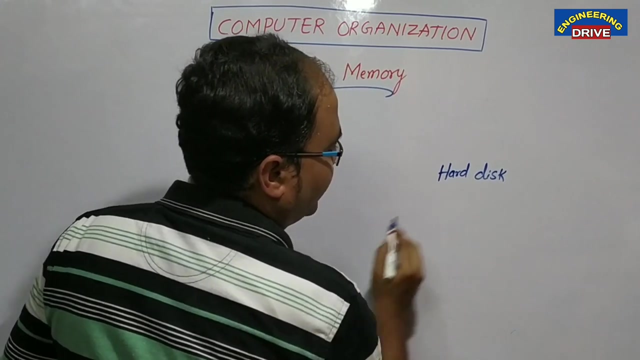 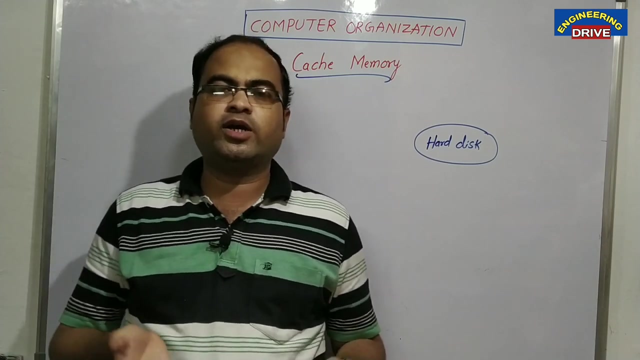 processor. you can understand with this simple diagram now. okay, so whenever i install any software or any programs where they are stored first, they are always stored in hard disk where those programs are stored. all those programs are stored in my hard disk either in c drive- generally in our computer c drive- or, if we take a the example of smartphone, in internal memory. 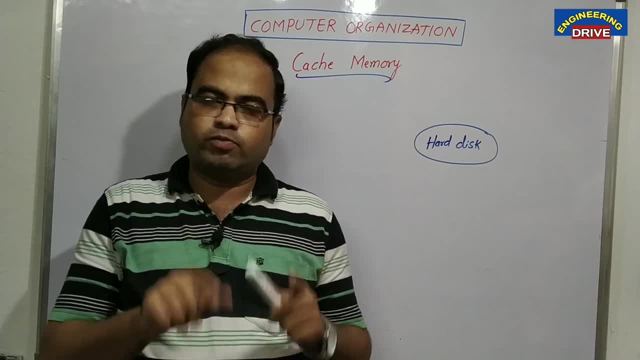 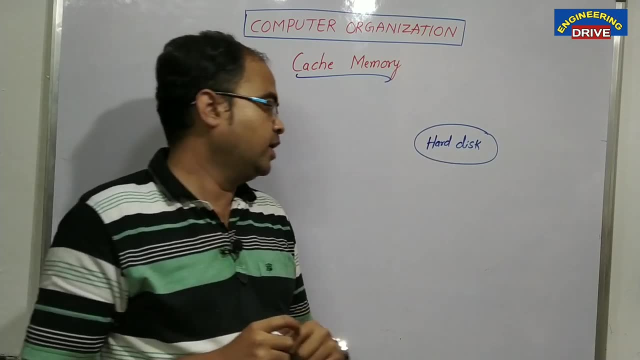 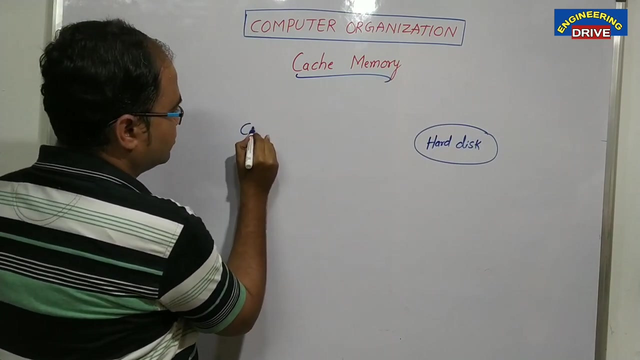 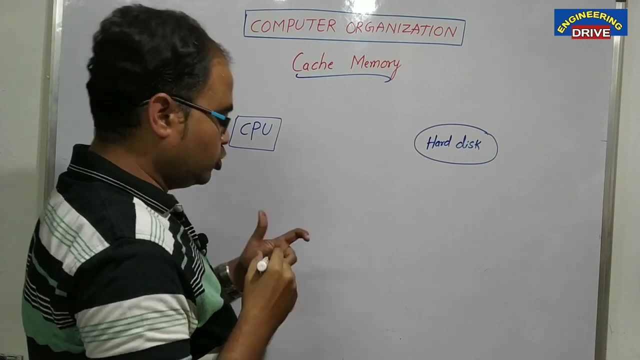 okay, so let us say i have installed one software. software means collection of programs. program is set of instructions. that entire software is loaded in hard disk. now, okay, now this is hard disk. this is the place where our programs are there. now here is our cpu, who need to execute those programs first. our cpu should execute those programs. a. 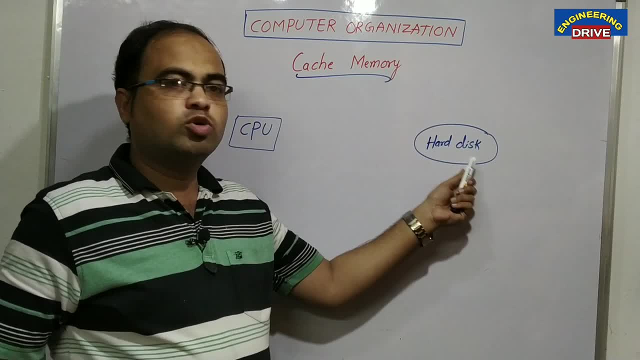 programs means instruction. wise, our cpu should execute those instructions now. but the rest, all of those things, if our cpu either this hard disk run in cont方面 and also, and cpu should execute those other programs, will not be safe. consuming that history that it is much easier. 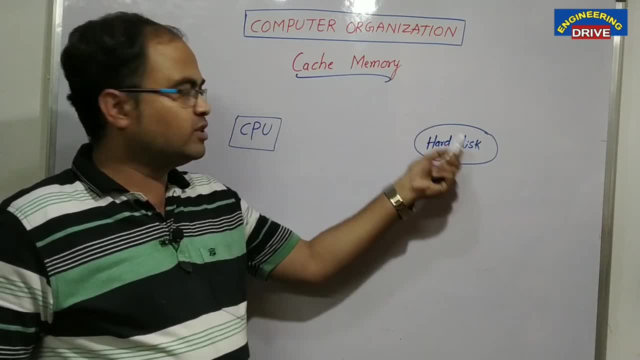 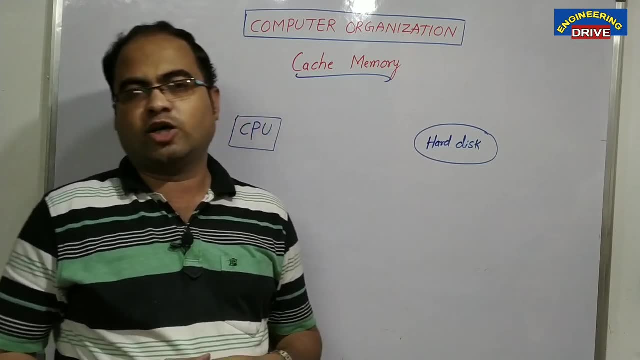 Where those instructions are available In hard disk. So directly, can our CPU will take those instructions. No, it is not possible Directly can our CPU will go to hard disk and execute the instructions. No, it is not possible. Then what our CPU will do. 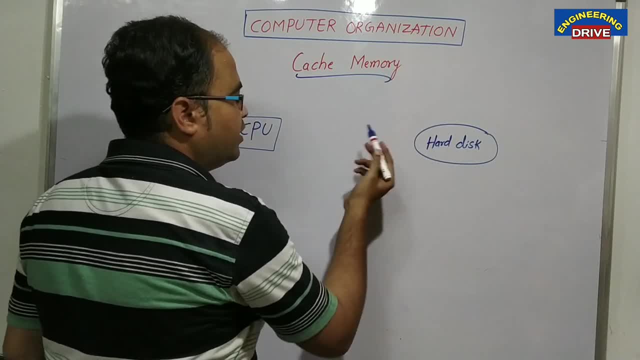 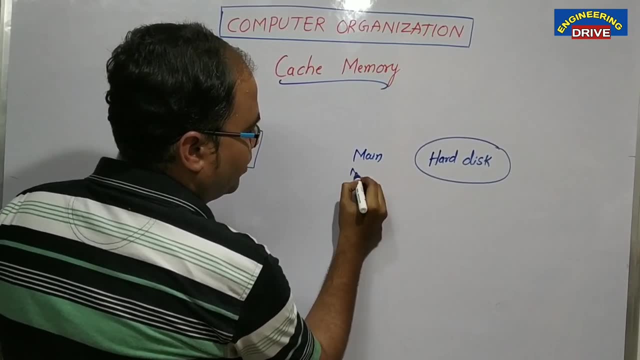 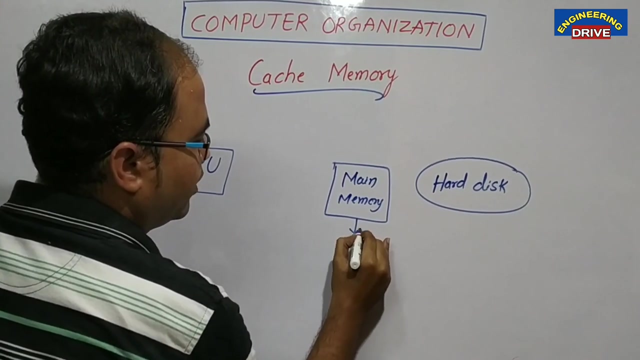 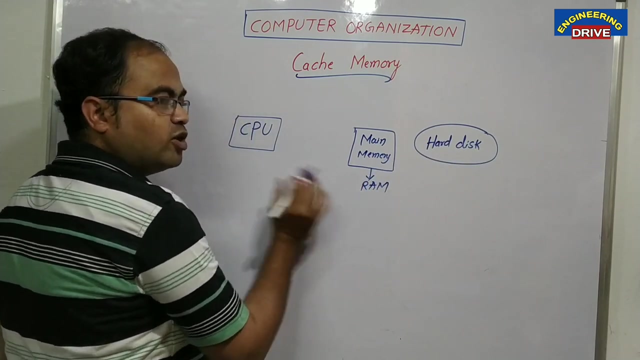 In between CPU and hard disk, there is one important memory known as main memory. What we call this one? We call this one as a simple way, random access memory. So the size of hard disk is larger or the size of RAM is larger. 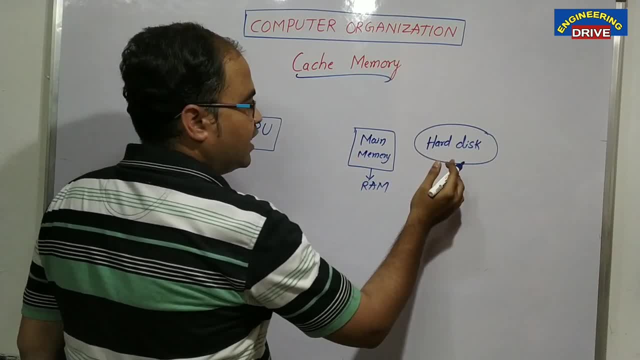 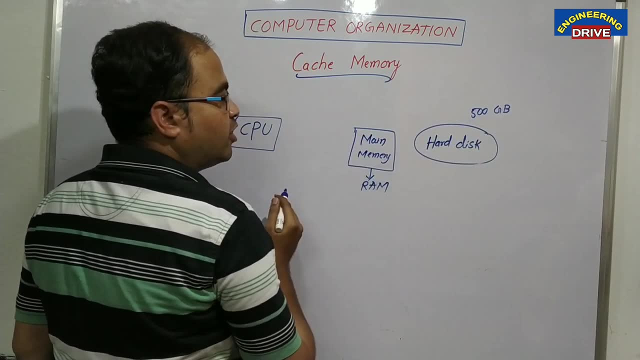 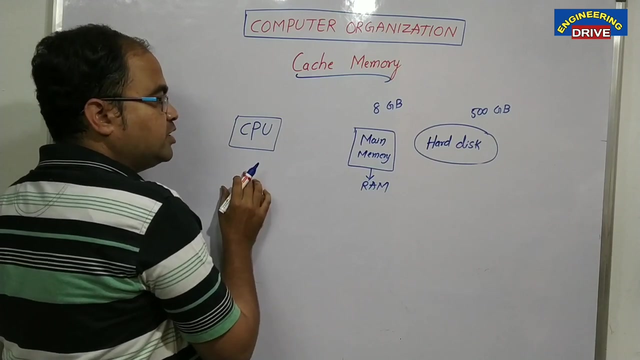 Of course the size of hard disk is larger. Let us say the size of our hard disk is 500 GB, Then what is the size of our RAM now, generally? Let us take the size of our RAM is 8 GB, Then what our CPU will do. 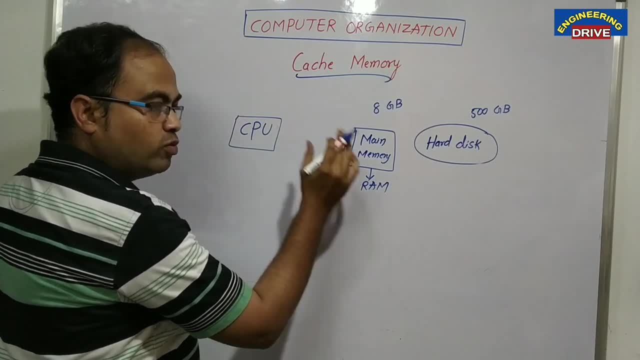 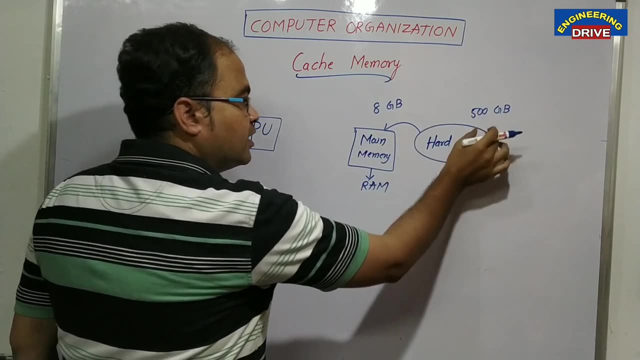 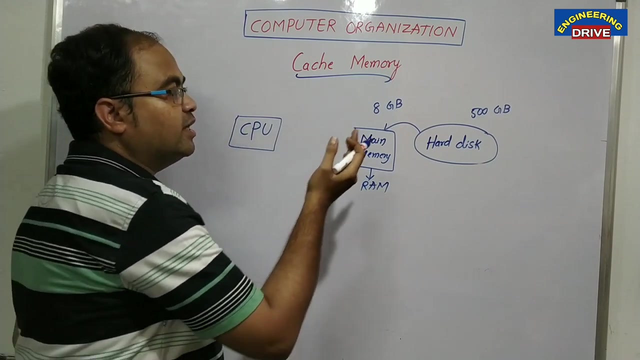 Suppose, if our CPU wants to execute one instruction, then CPU will take the instruction from hard disk. From hard disk it is brought into RAM Means. let us say if our program size is, or if our software size is, let us say, 140 GB. 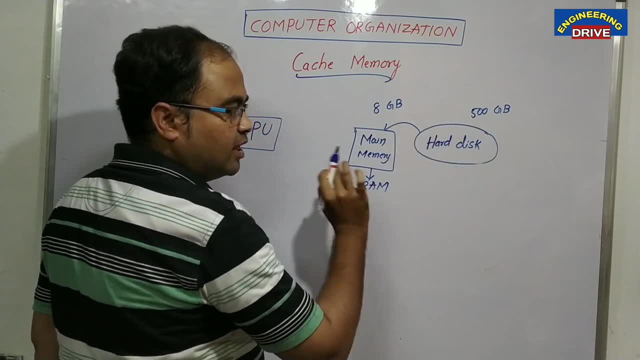 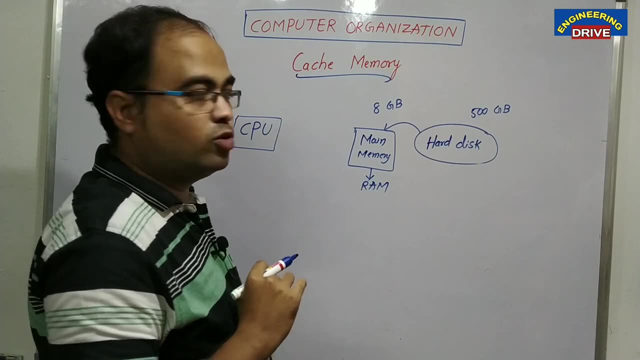 Example: very large software, 40 GB capacity, is there. It won't take that 40 GB because that 40 GB cannot be adjusted in this 8 GB. So whatever CPU will do, It will take only the necessary part from the hard disk. 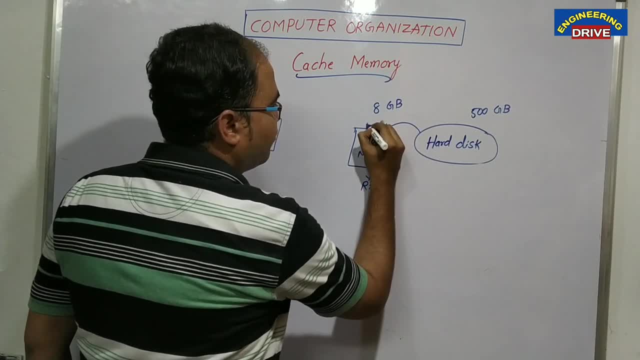 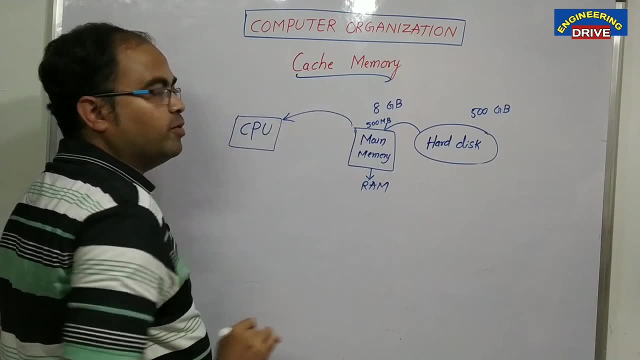 So let us say the necessary part is only 500 MB. It will copy only the 500 MB And that 500 MB will be taken by our CPU And then the instruction will be executed. Hopefully it has been clear to you. 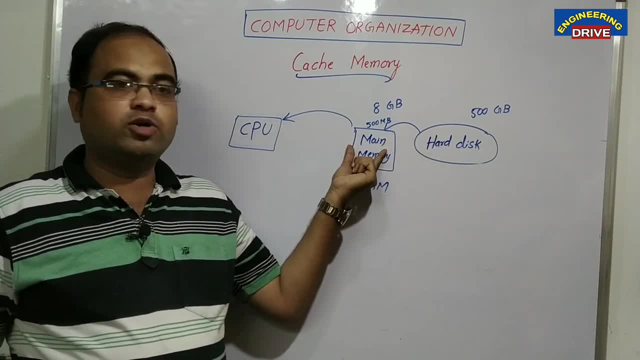 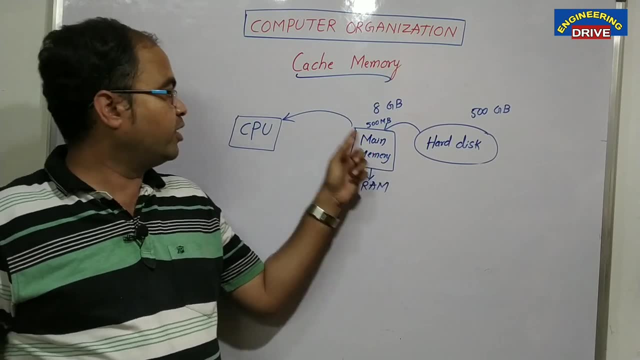 Initially the data will be stored in hard disk. From hard disk it is brought into main memory or RAM. Whether the entire programs are brought, No only the necessary part is brought into RAM. from RAM it is brought into CPU and CPU will execute that one. 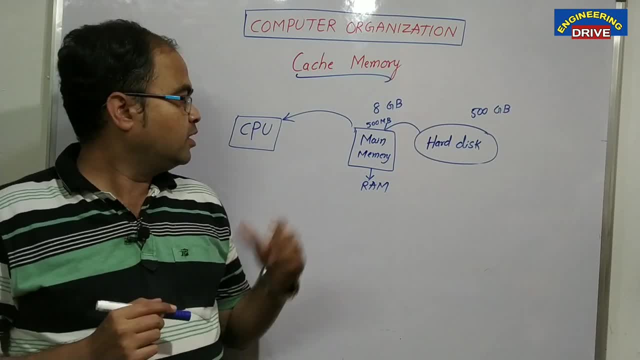 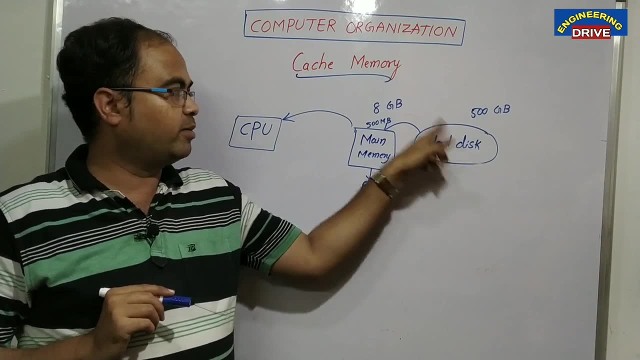 Okay, now the question that comes in our brain is now: if CPU want to execute second instruction, what CPU will do? Again same process: it will go to hard disk. from hard disk it is brought into main memory. from main memory it is brought to CPU. 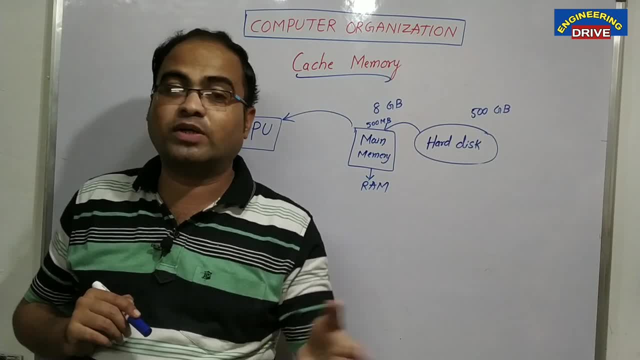 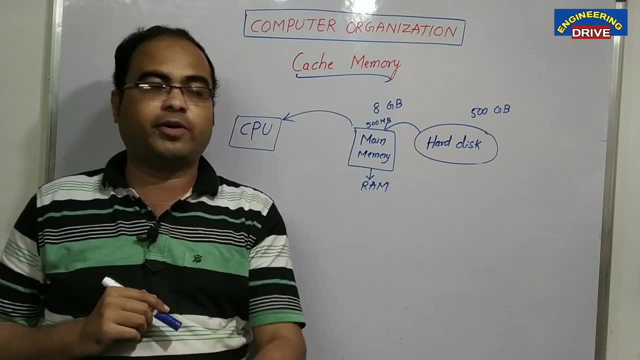 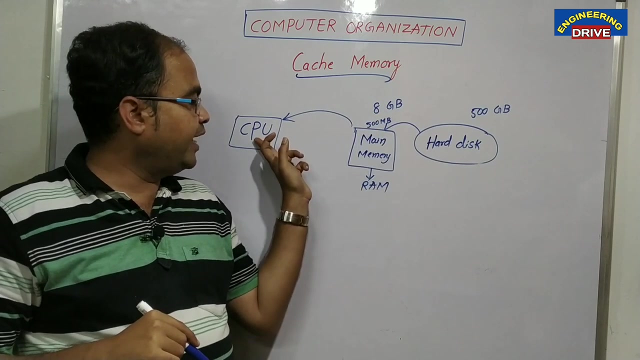 Okay, if CPU want to execute instruction number once again now, second time, then what CPU will do? Whether it will search the data from hard disk again. No, this is very, very important point. If CPU want to execute instruction one once again, instead of going to hard disk directly, it will take the data from main memory only. 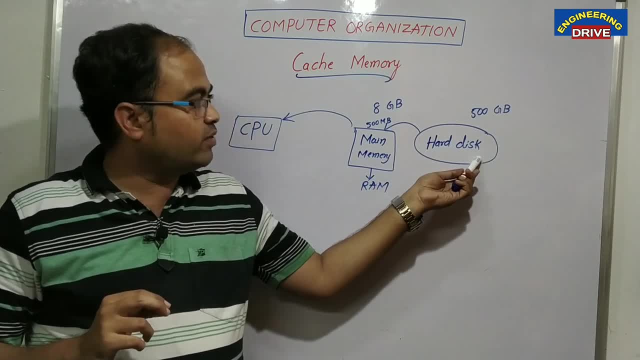 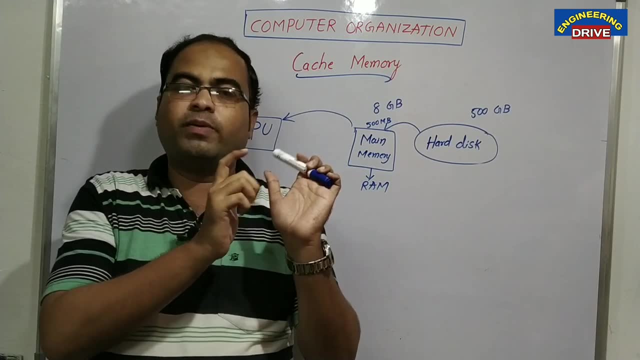 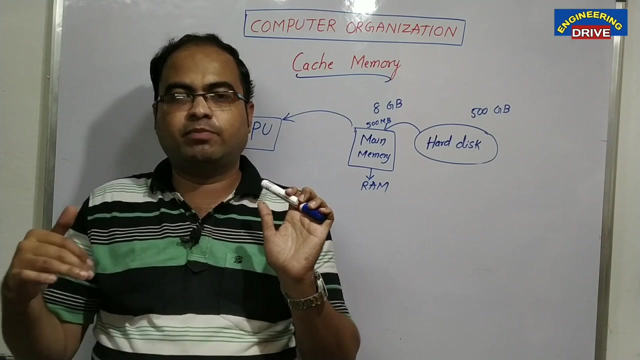 Why it will take the data from main memory? Because that instruction one is already available in RAM, that is, in main memory. Even if we take the example of our smartphone also, you open one application in your smartphone, Okay, and you just press back button from your mobile phone in standby mode. 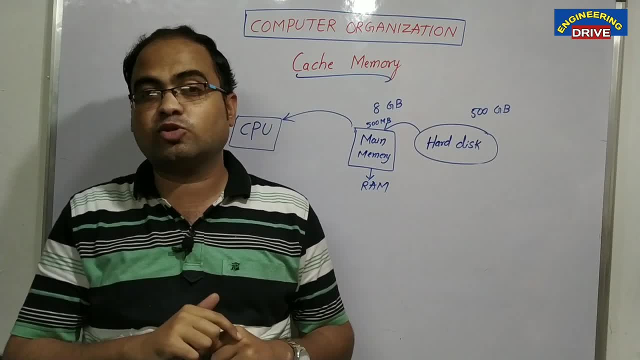 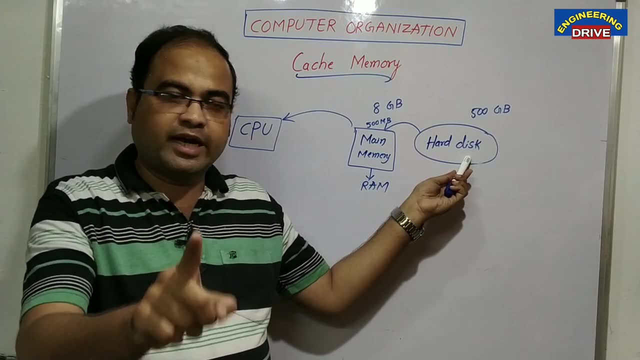 Again, you go and open the application. Whether the application will open fast or slow, it will open compulsory fast. Why it will open compulsory fast? Because already you have opened. when you open the application first time, it will copy it from your internal memory or hard disk and it is brought into RAM. 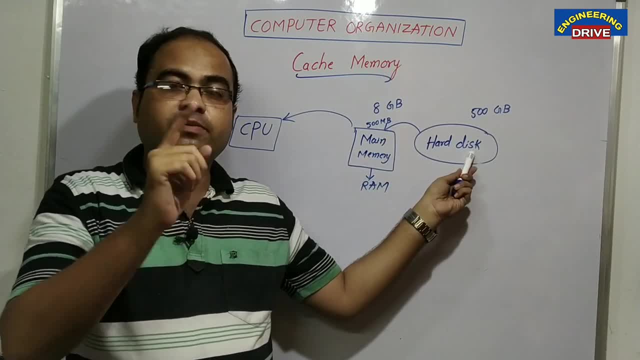 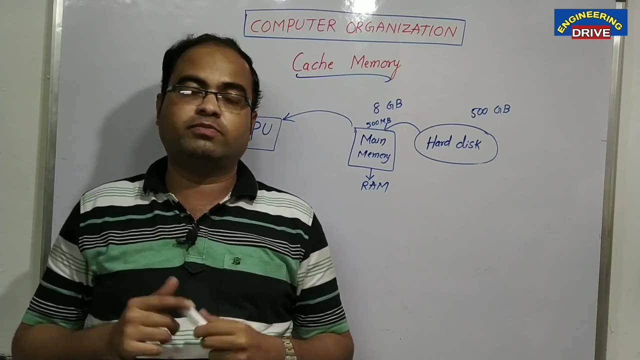 When you open for second time, our CPU won't search that program or instruction in the hard disk Directly. it will take it from the RAM. That is why it will open very fast to you, my dear students. Same thing happening here also in our computer. 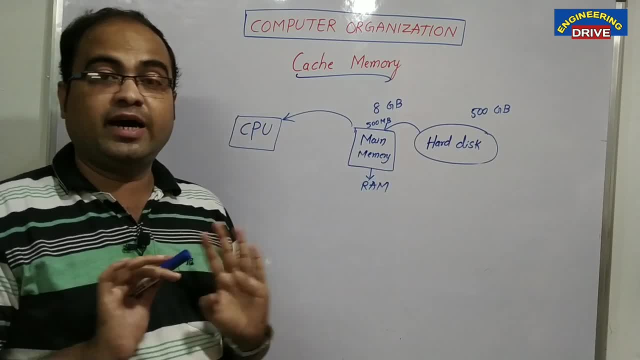 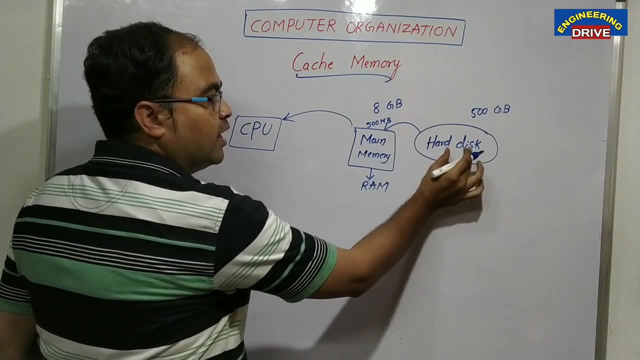 Okay now, whether case Memory is available here. No, still I have not discussed about case memory now. Now, this sequence is okay, But the problem with this sequence is the speed of hard disk is very slow. Next, the speed of main memory is somewhat fast. 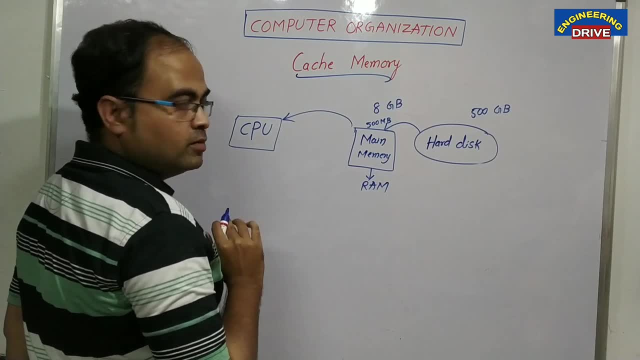 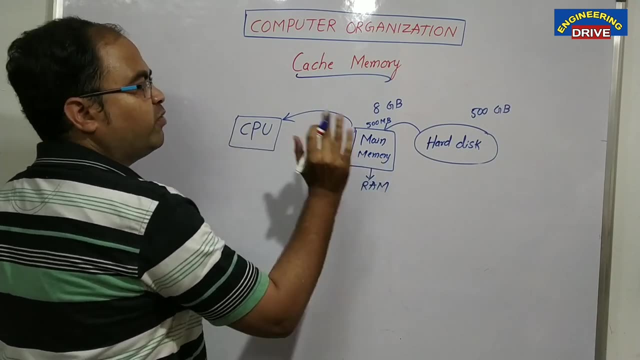 No problem, And the speed of CPU is very fast, Which means there is some synchronization problem between CPU and main memory, Because the speed of CPU is very fast, Tremendous, Whereas the speed of main memory is fast, Fast but not so fast compared to CPU. 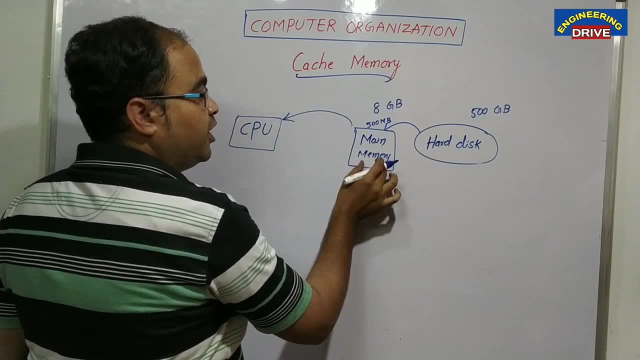 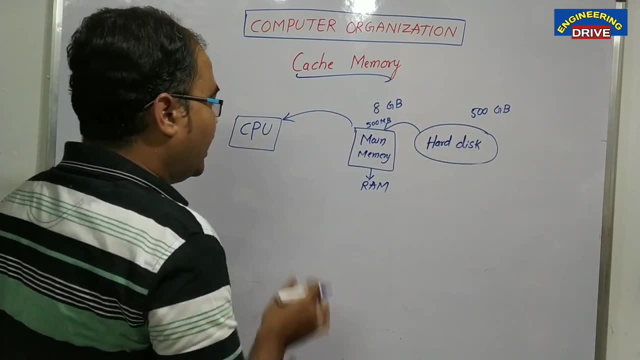 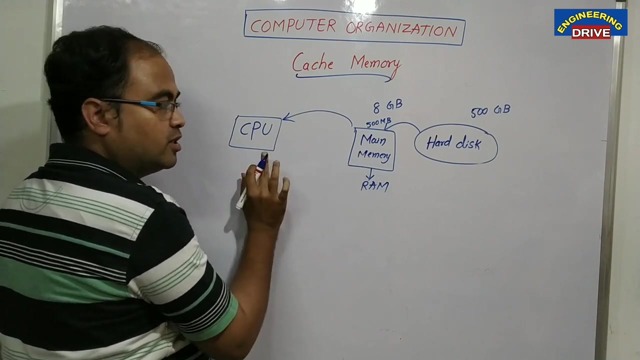 When we compare main memory and hard disk, the speed of main memory is fast compared to hard disk, So which is very slow. in this one, hard disk is very slow. So what we are doing here means CPU and main memory. their speeds are. we are not able to match their speeds. 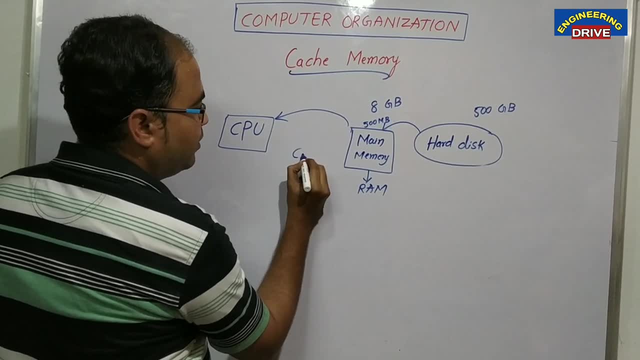 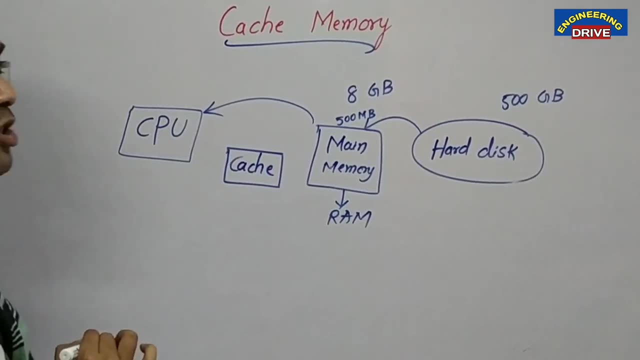 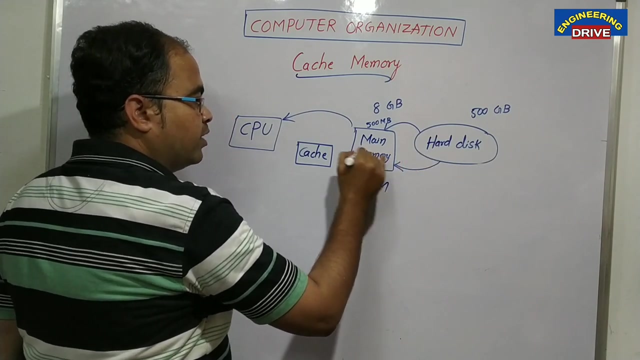 So because of that, in between CPU and memory we are keeping one small amount of fast memory. We call that small amount of fast memory as case memory. So what happened First? the instructions will be brought from hard disk to RAM. 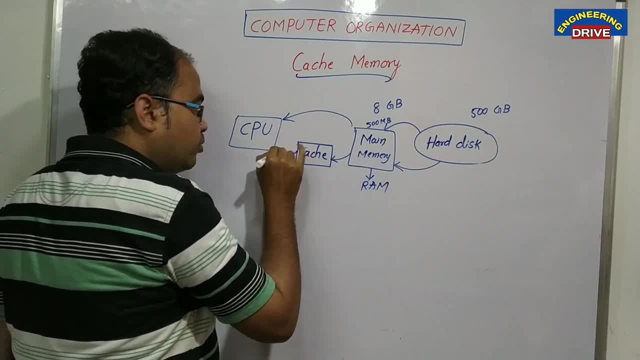 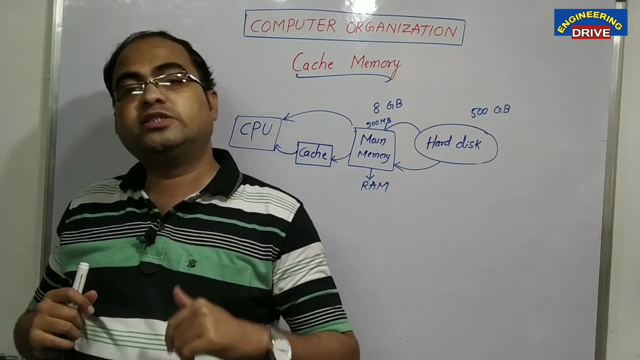 From RAM it is brought to case memory. From case memory our CPU will take the instruction And it will execute the instruction. Then, if the CPU want to execute the same instruction second time, what happened? CPU won't search that instruction in main memory. 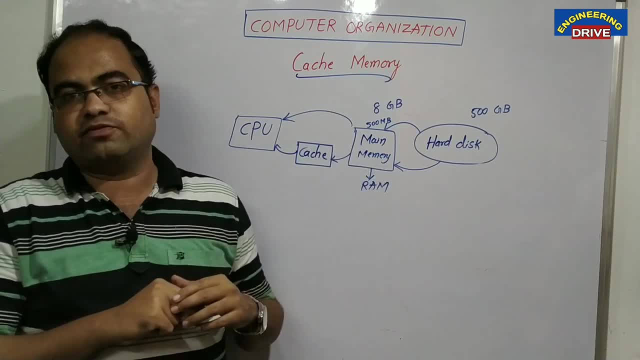 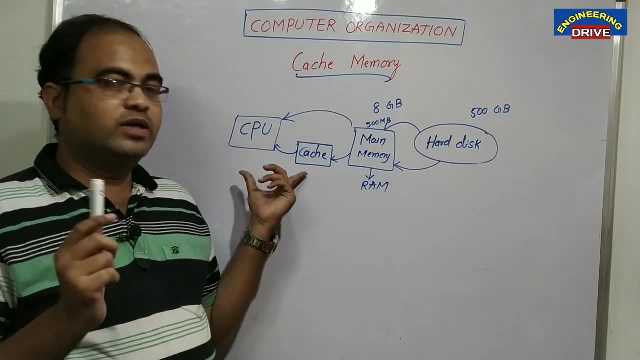 Instead of main memory, it will search the instruction in case memory itself. So what will happen? CPU easily can find the instruction. It can execute the instructions very fast. So once again, I am saying to you, the size of hard disk is very large. 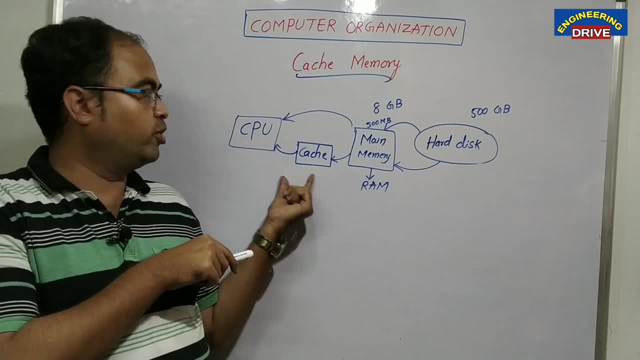 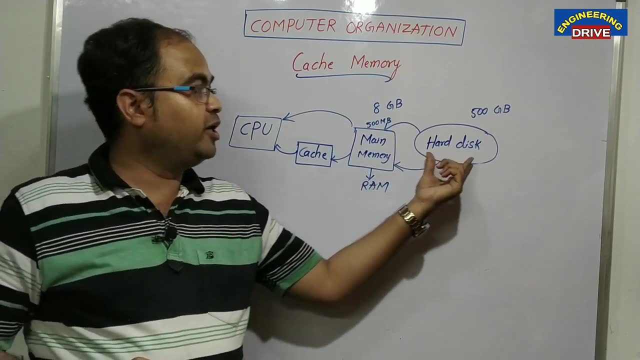 Next, smaller one main memory, Next smaller one case memory. And the size of CPU is very small compared to this four. Now we are talking about speed. The speed of hard disk is very slow. The speed of main memory, or RAM, is faster. 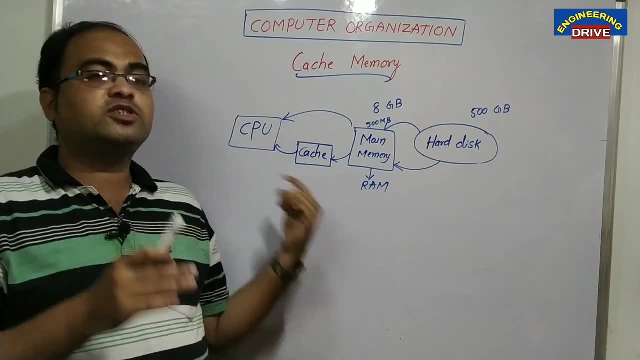 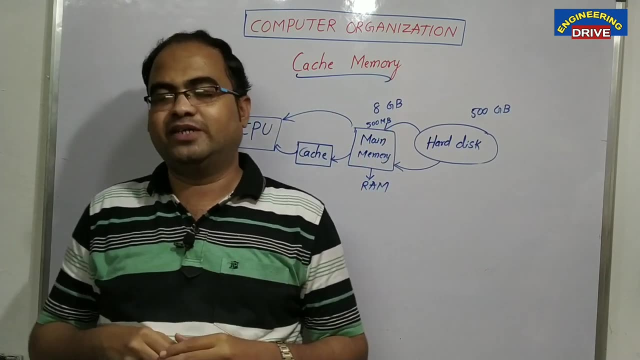 The speed of case memory is very fast, Whereas the speed of CPU is tremendously fast, Which means they are reversed when compared to two qualities: Sizes and speed. Okay, my dear students, So this is the working of our case memory. 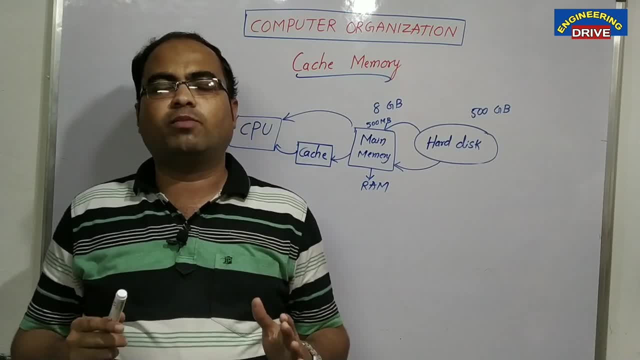 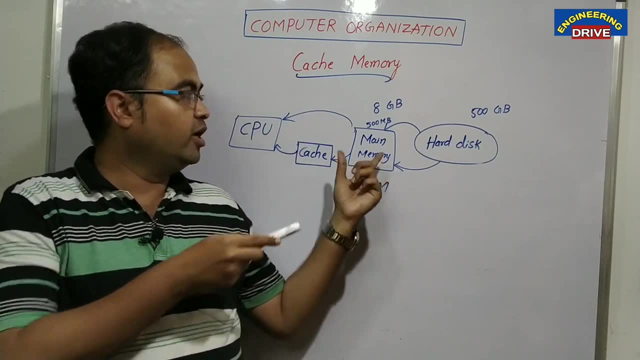 What is case memory? Case memory is a very small amount of fast memory Which is mainly used to increase the transfer speed between CPU and main memory. If you want to increase the transfer speed between CPU and main memory, we will keep on case memory. 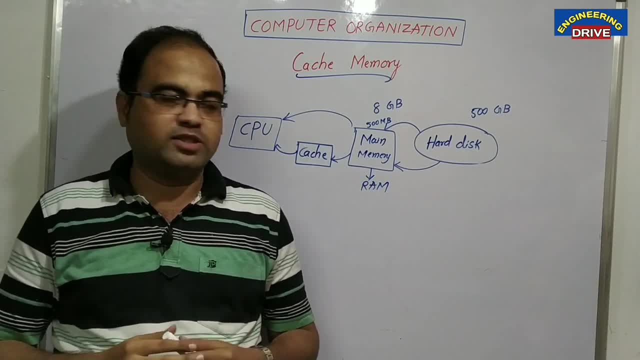 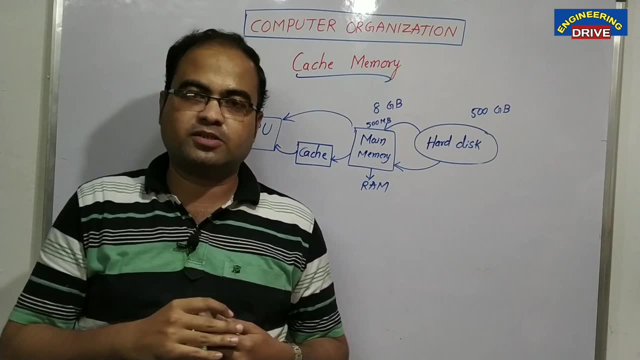 At last with one real memory For real time example, I will close this concept. Let us say you are in a class One faculty came and asked you bring chalk piece. One of your teacher entered in the class And the teacher asked you one class representative or one student? 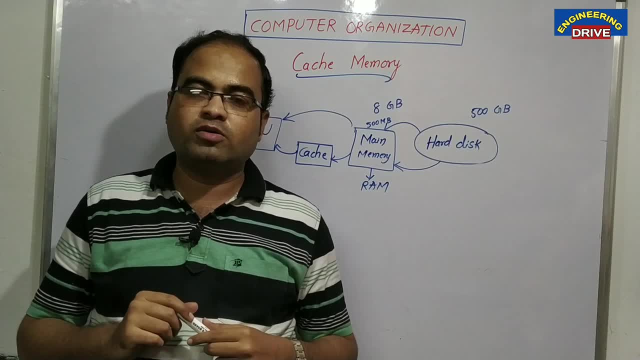 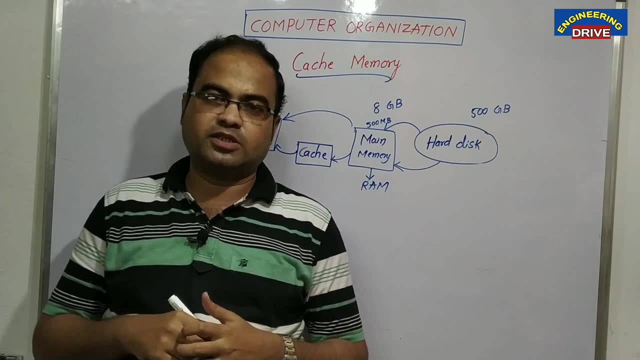 Yes, go and bring chalk piece. Then what the student will do, From where he will get the chalk piece, He will directly go to staff room first, Because in staff room we will keep the chalk pieces. So let us say, in staff room also, chalk piece is not available. 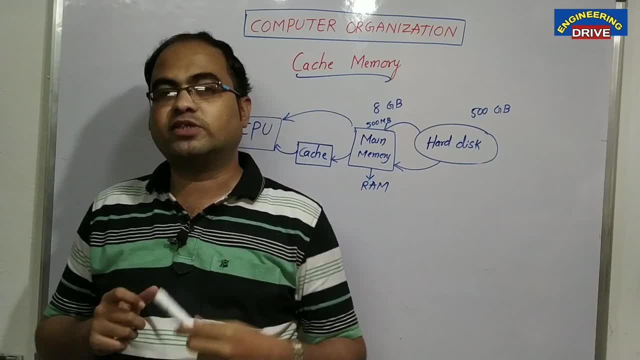 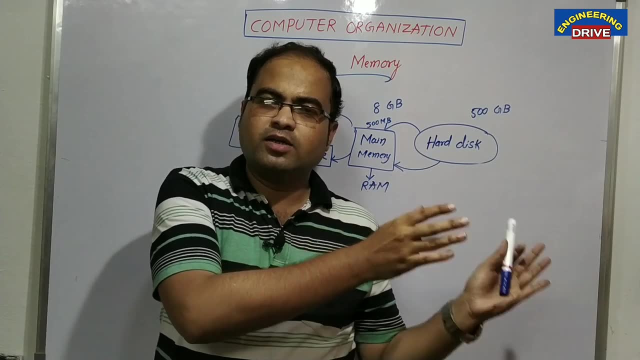 Where the student will go now. He will go to office of that college, Yes or no. Which means, let us say, chalk pieces are available in staff room itself. Then what happened Second time? student will not go to office directly. 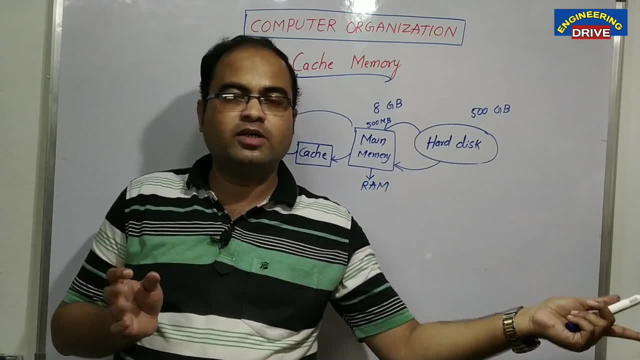 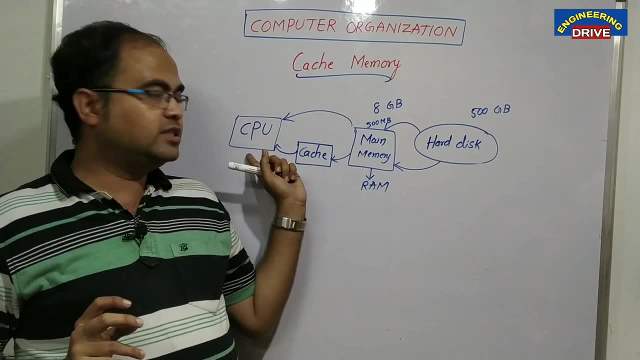 Student will take the chalk pieces directly from staff room itself. So you can take the example: office as a hard disk, Staff room as a main memory And CPU as your classroom. Now what I am doing? Same work. I am reducing the time now. 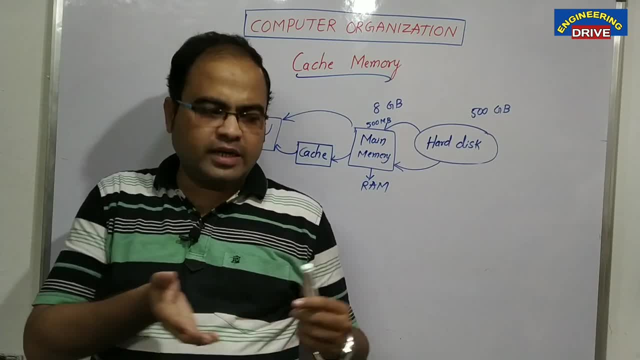 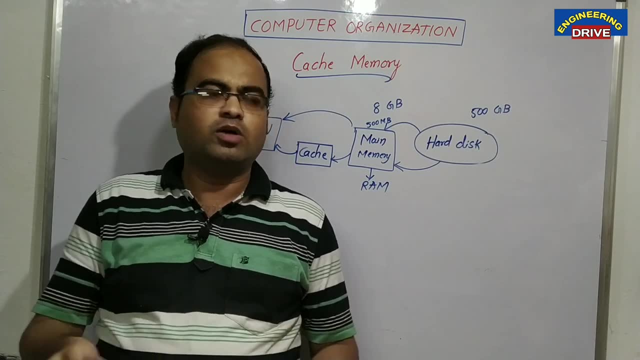 Which work, Why you are going to staff room also. Keep the chalk pieces. beside your class itself. There is one small store room. Keep there only Why you will go to staff room also. So which means that small store room beside your classroom is your cache memory. 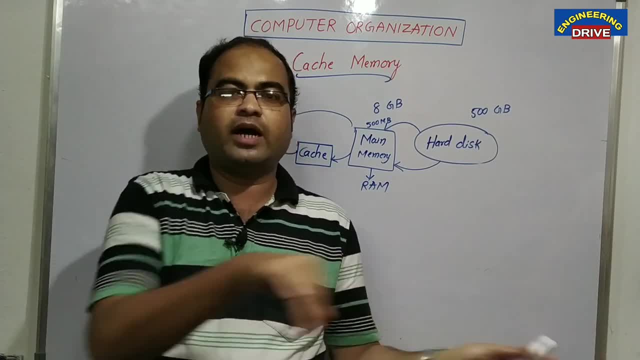 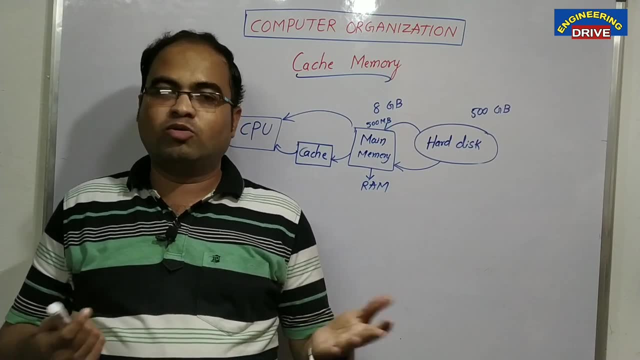 Okay. So whenever you want chalk piece directly you can go and have that chalk piece. So the work of going to staff room- that is main memory or hard disk- will reduce. Okay. So hopefully The use of cache memory has been clear to you.